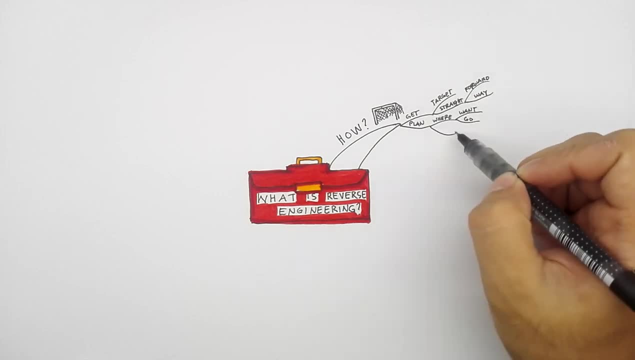 You need to plan where you want it to hit inside of the goal and you kind of retrace the steps for where it hits the goal back to where you are. Imagine you've got a bike and someone tells you to assemble a bike and you've got a diagram with all the parts and your job is to assemble it. 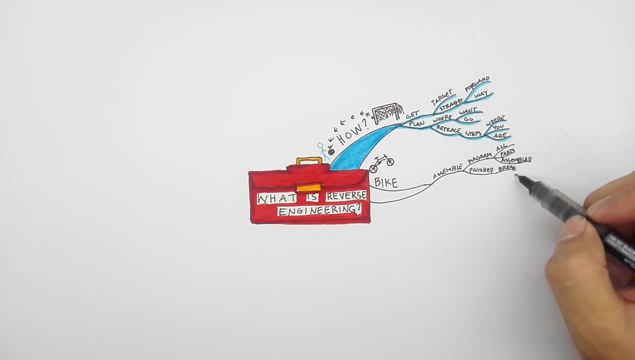 But also imagine you were given a finished bike and you got to break it down completely and then put it back together. It's easier to put the bike back together rather than just starting, And it's the same with getting results for an exam. You need to break down what you need to do. 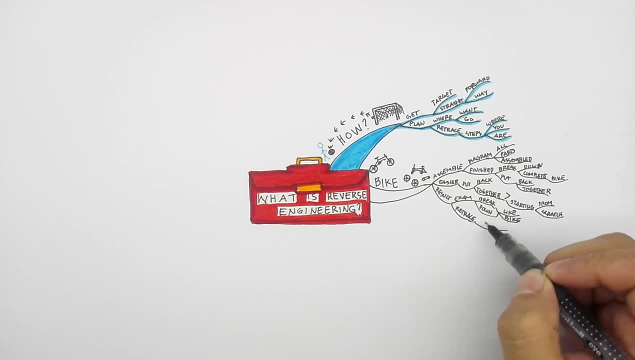 to get to the exam like the bike, and retrace your steps and imagine those steps and imagine you're kind of putting the bike back together again. So what I'm trying to get you to do is to visualize the steps from a lesson to an exam, to get you back from the exam to your current place. and to get you back to where you are. So what I'm trying to get you to do is to visualize the steps from a lesson to an exam, to get you back from the exam to your current place and to get you back from the exam to your current place and to get you back from the exam to your current place. 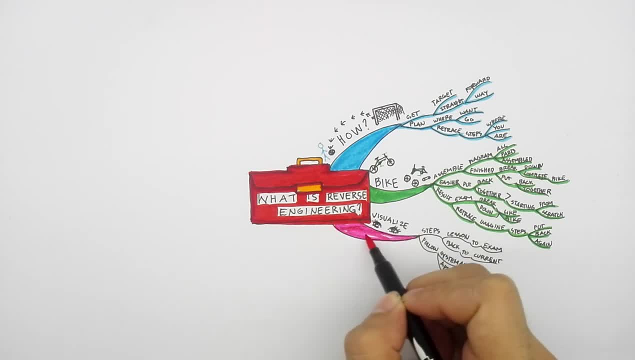 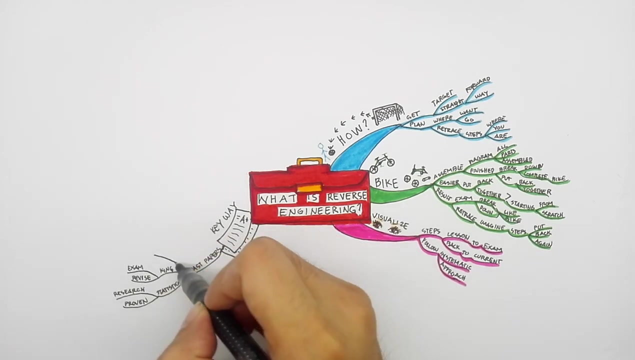 And to do that you need to follow a systematic approach, like putting the bike together again, And one of the key ways of doing this is using past papers. It's statistically proven with research. It's the king of revision for exams. When you do a past paper, it helps, you know. 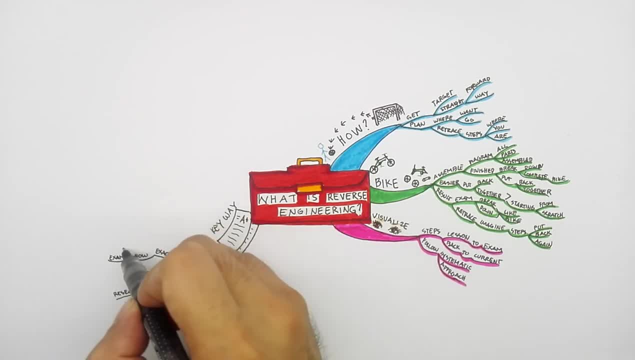 exactly how you're meant to answer that exam And it also helps you imagine doing a real exam. Research has shown that the more past papers you do, the more chance you have of doing well and getting better results Now with a mind map. 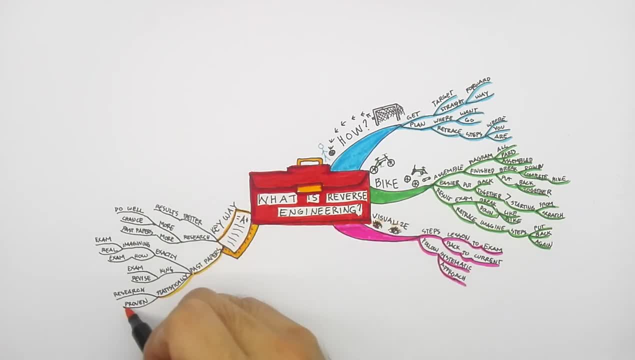 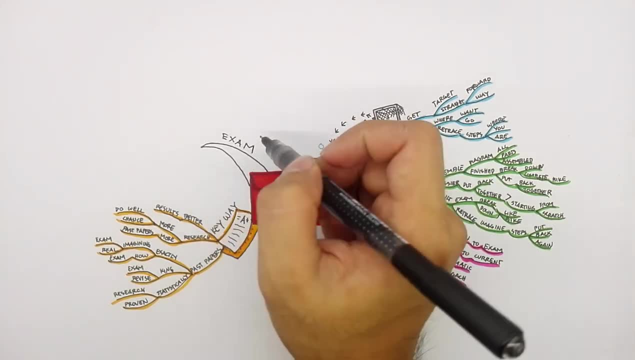 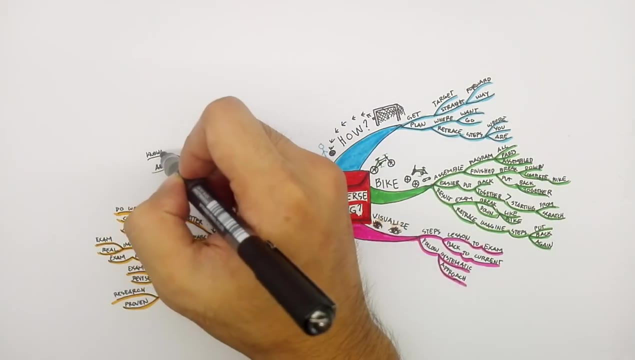 you can answer past papers more rapidly than just writing an essay. It can take you an hour to write an essay for an exam as a practice, or 10 minutes to do a detailed mind map outline. Remember an exam is not just about knowing the whole subject. They're trying to see how much you can.